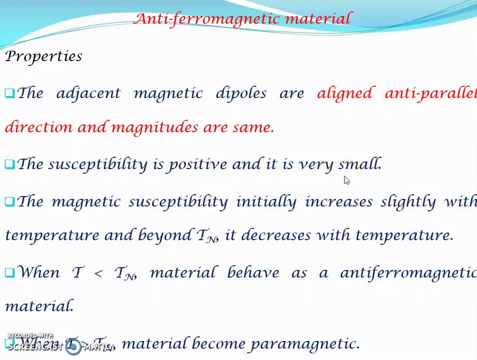 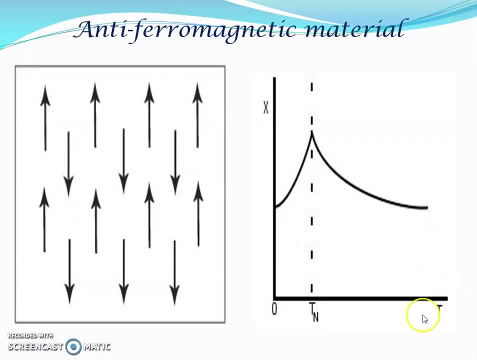 Susceptibility is positive and the susceptibility value is small in the case of antiferromagnetic material. Then just see The graph: temperature along x-axis and susceptibility along y-axis. As temperature increases, susceptibility also increases and reaches maximum susceptibility at a temperature. 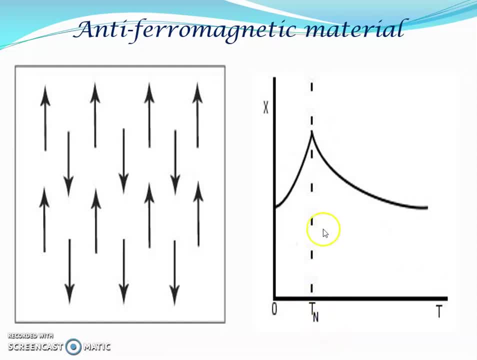 called nil temperature, Tn. Once nil temperature is reached, still if we increase the temperature, the magnetic susceptibility starts decreasing. So nil temperature, Tn, nil temperature, Tn temperature is the temperature at which the susceptibility is maximum in the case of 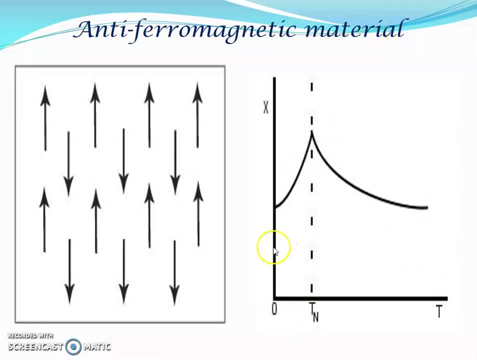 antiferromagnetic material. So below nil temperature susceptibility increases and above nil, temperature susceptibility decreases. So we say that when T is lesser than Tn, that is this portion, we call it as antiferromagnetic material. When T becomes greater than Tn- this portion, the material becomes paramagnetic material. So these are the 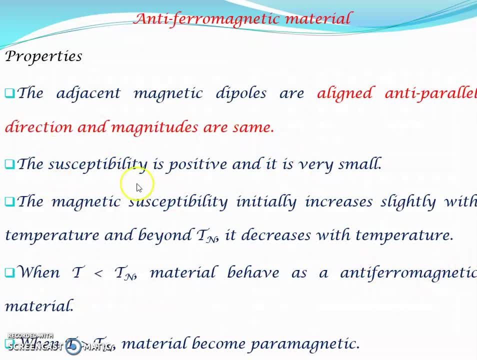 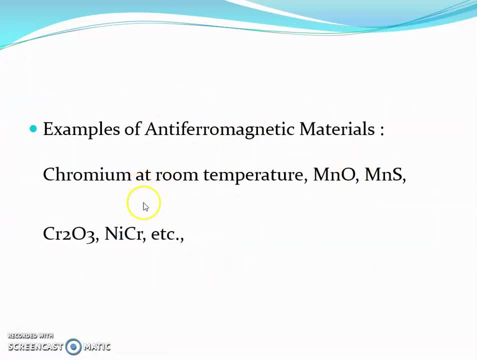 properties of antiferromagnetic material. Examples of antiferromagnetic materials include chromium at room temperature, manganese oxide, manganese sulfide, chromium oxide, nickel, chromide, etc. Next ferrimagnetic material are the properties of antiferromagnetic material. So these are the properties of antiferromagnetic. 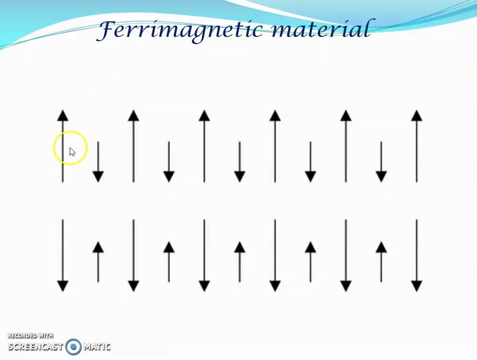 material otherwise known as ferrite. So if we see the dipole, alignment, adjacent dipoles, they also point in antiparallel direction, but their magnitudes are different. So see here, from here to here, we have, but if we take the adjacent dipole, the magnitude is going to be different. 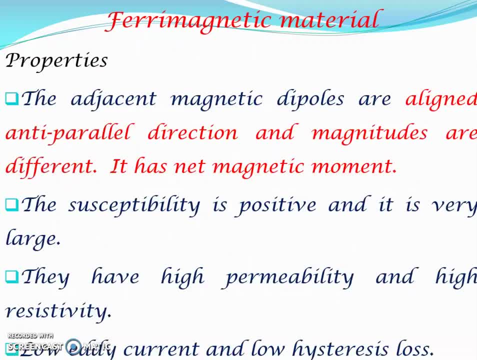 from this one. So the properties of ferrimagnetic material include the adjacent dipole moments are aligned, antiparallel direction and magnitudes are different. It has net magnetic moment, The susceptibility is positive and it is very large. They have high permeability and high resistivity.